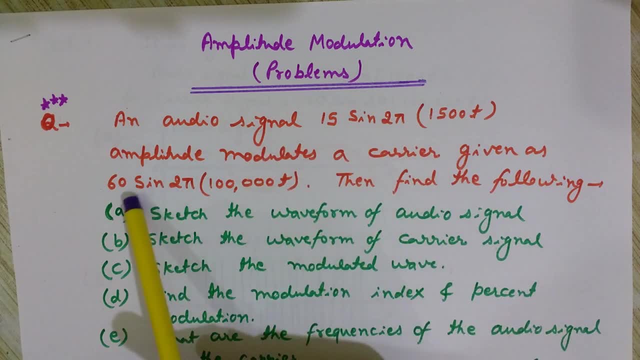 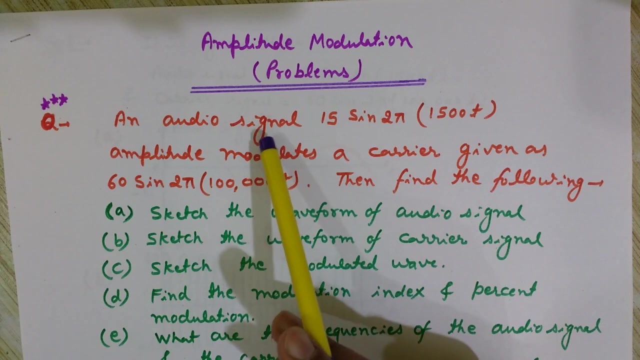 a carrier wave. this carrier wave is given by 60 sine 2 pi, 1 lakh. this is 1 lakh, actually 100000 T. then find the following: we will calculate all these things here we are given with the audio signals equation, The message signal that you want to transmit and the carrier wave equation that is being 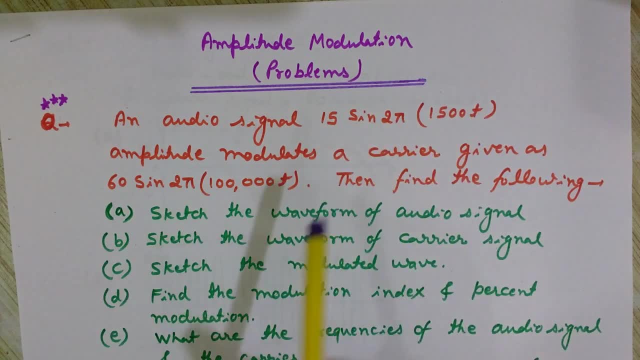 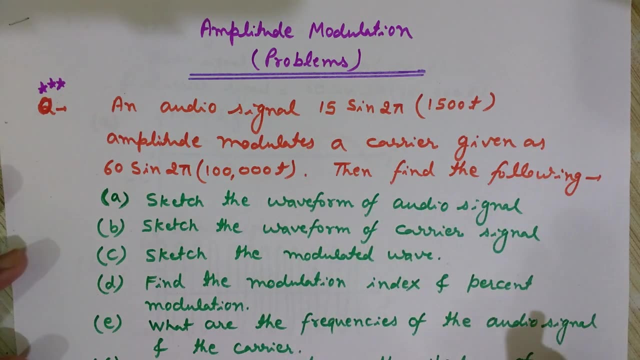 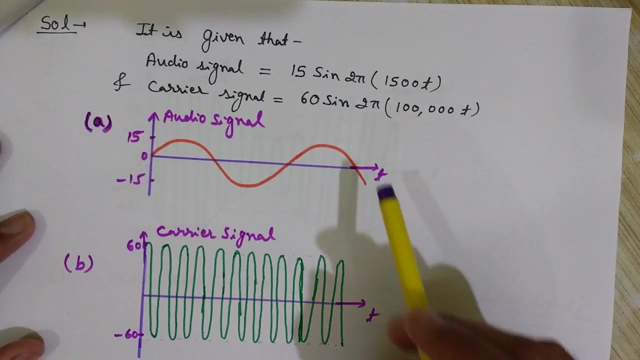 modulated by this audio signal. so let's find all these things. first is sketch the waveform of the audio signal. let's now sketch the waveform of the signal. this is the equation of the signal: 15 sine 2 pi, 1500 T. you see here, this is the waveform of our audio signal, our audio. 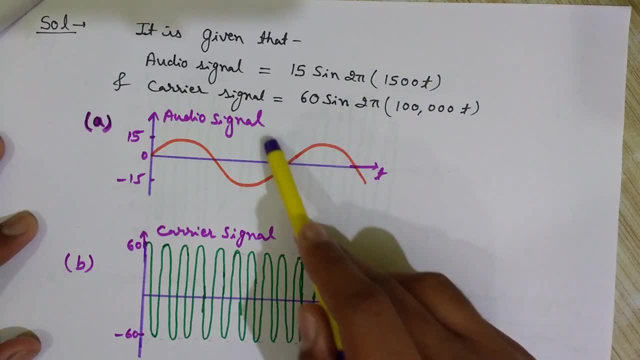 signal is given by this And this is the carrier signal. So this, you can see that this is a sinusoidal signal, so the sine wave, we know. this is the shape of the signal and what will be its amplitude. its amplitude will be 15 because the standard 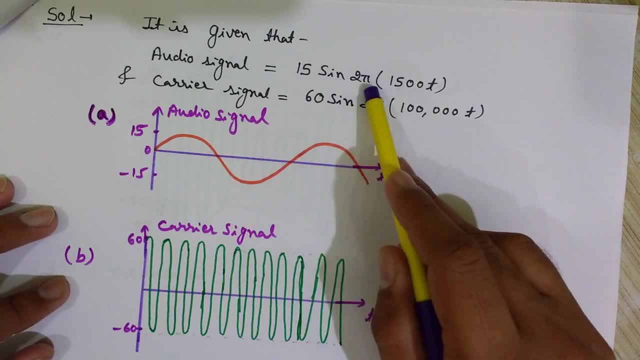 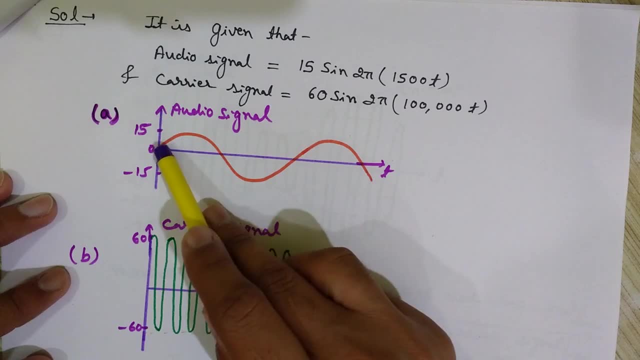 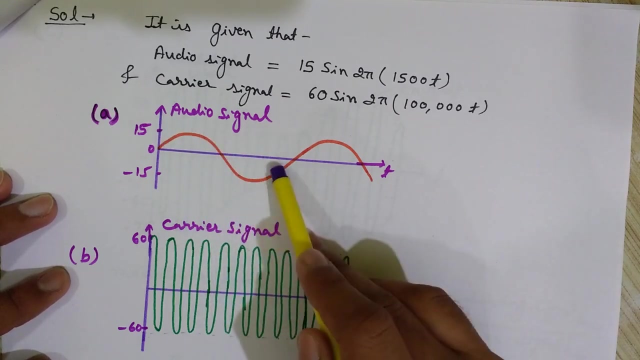 format for this equation is a sine of 2 pi f into T, so a is the amplitude maximum peak value, so 15 is the amplitude. you see here, it is a sinusoidal wave and its amplitude is 15.. So This is the positive peak and this is minus. 15 is the negative peak. so it is very simple. 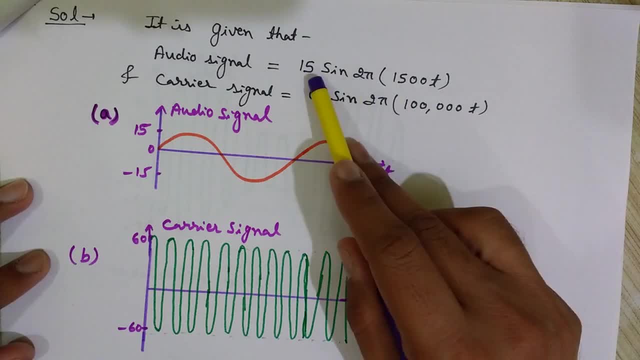 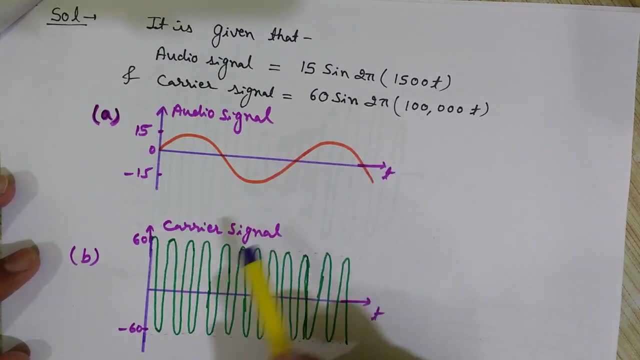 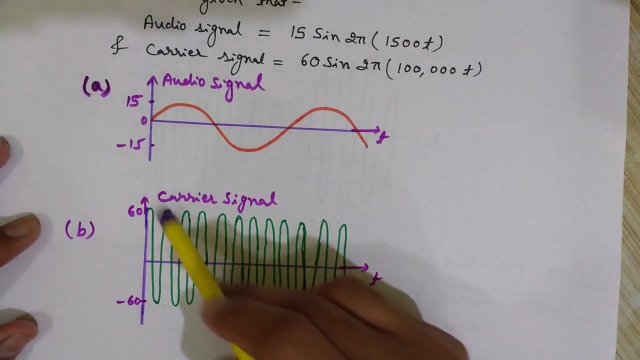 and its frequency is 1500 because its standard format is a sine 2 pi f into T. so f is this, this is frequency. Now let's draw the carrier signal. the second part is to sketch the carrier waveform. so this is our carrier waveform. you can also observe here that, as I told you that the frequency 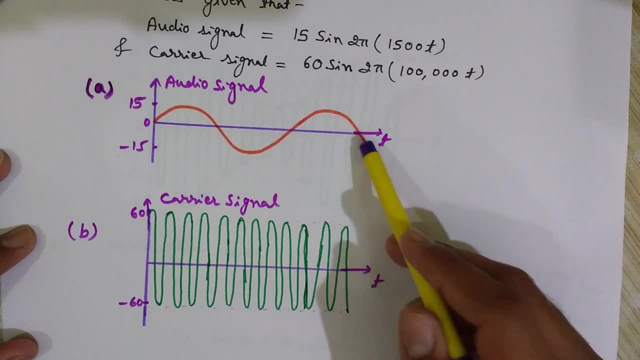 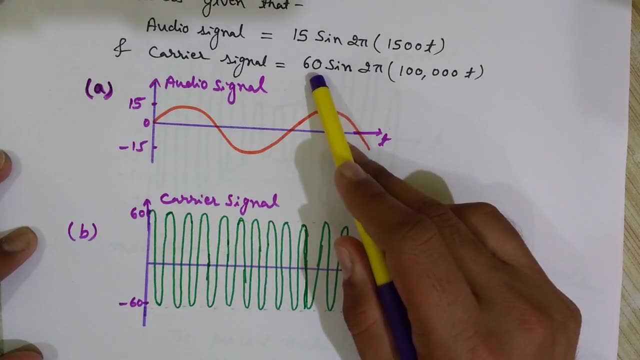 of carrier wave is very high In comparison to the modulating signal. so you see its high frequency. So what is the equation of carrier wave? it is 60 sine 2 pi, 1 lakh of T, 1, 0, 0, 0, 0, 0, 0 T. 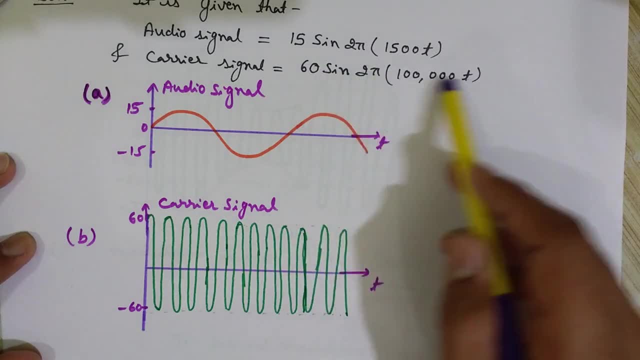 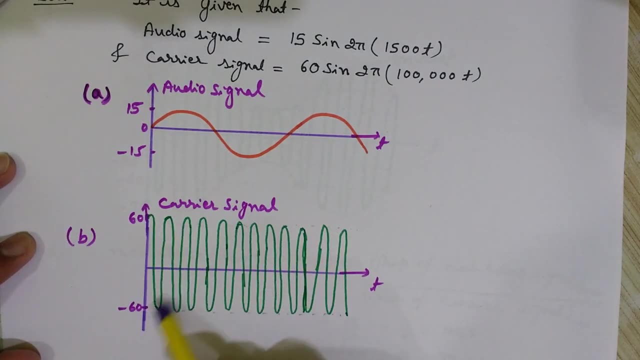 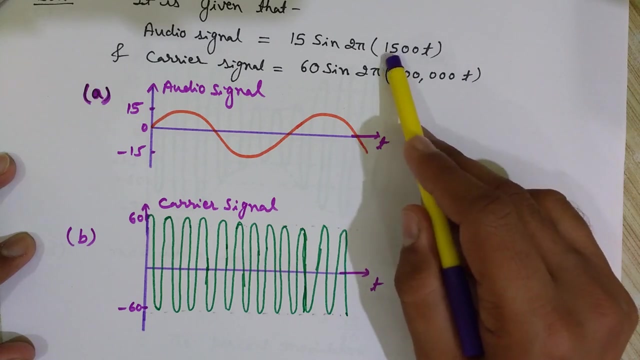 it is the amplitude 60 a sine 2, pi, f, T format. by this we have 60 as the amplitude positive side, 60 negative side. its peak value is minus 60 and it is also a sinusoidal graph and you can observe It, that its frequency is 1500, while its frequency is 1 lakh, or you can say 100 k, also clear. 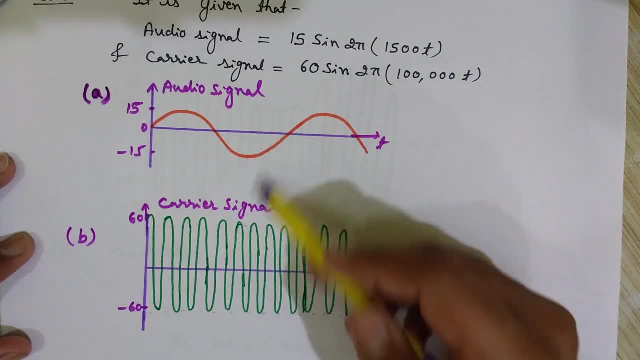 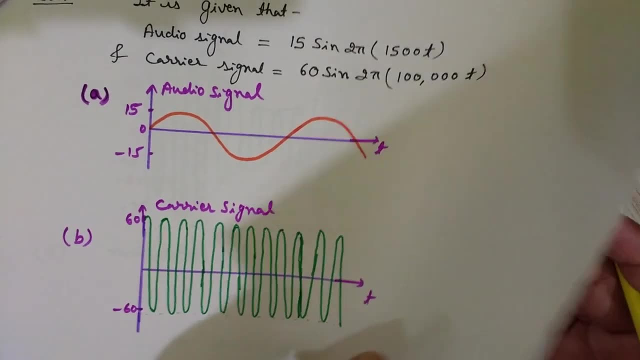 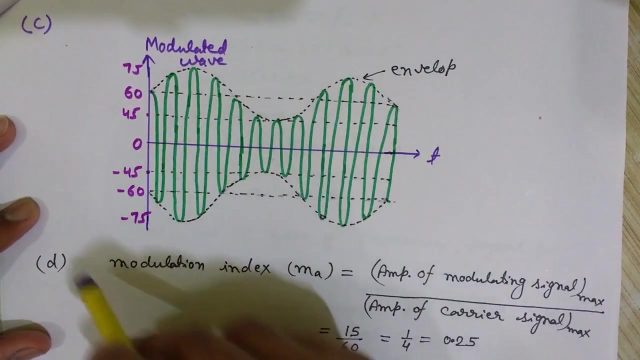 by this waveform, that its frequency is much larger than the, than this message signal, this audio signal. Now, third part of the question is to sketch the modulated signal. This is our modulated signal. how we get this modulated signal? Actually, We know that. as I told you earlier what is amplitude modulation in amplitude modulation? 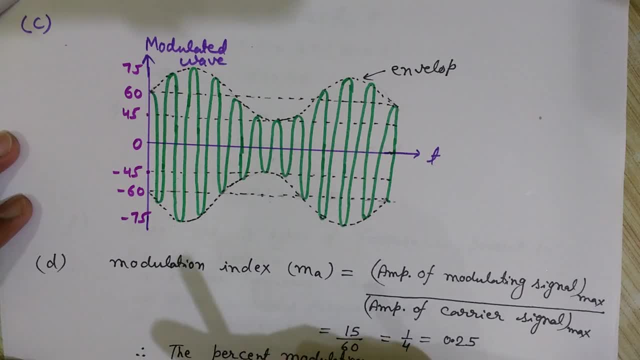 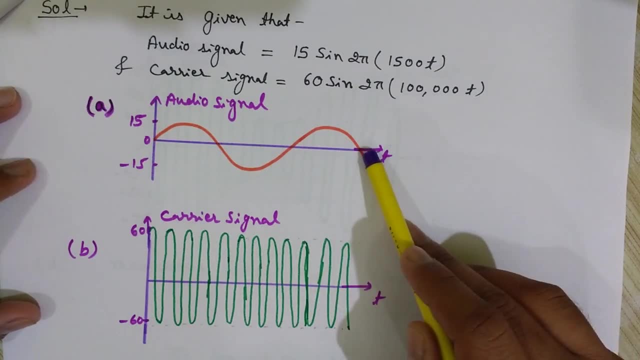 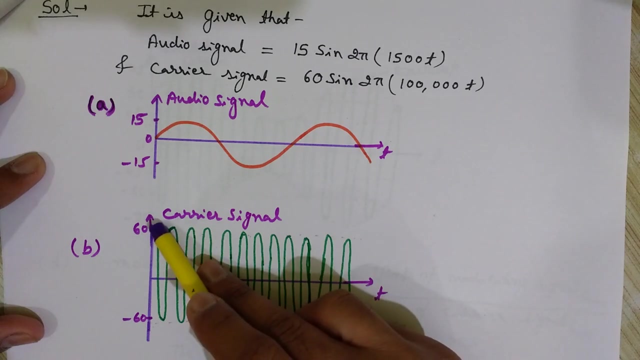 the amplitude of the carrier wave is varied according to the instantaneous value of the modulating signal. here This is the variation of amplitude of the message signal. OK, this is the shape of the message signal: audio signal. What we will do in amplitude modulation, we will change the amplitude of this carrier. 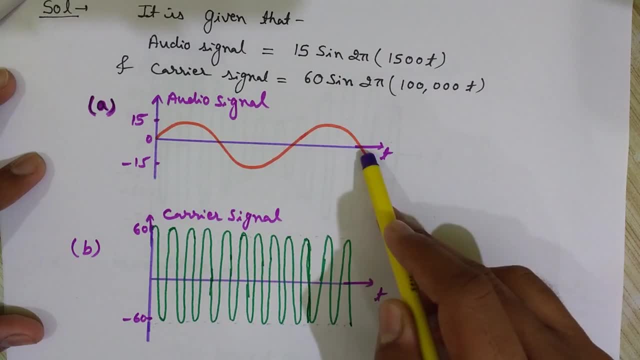 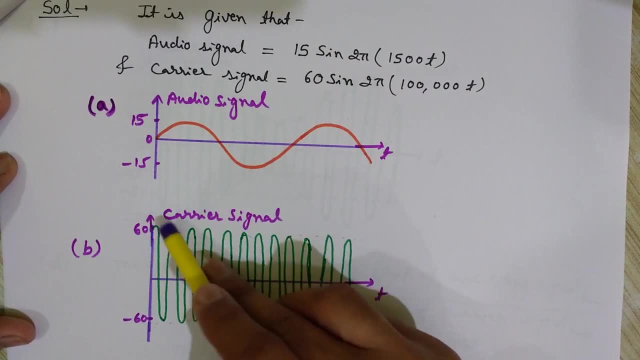 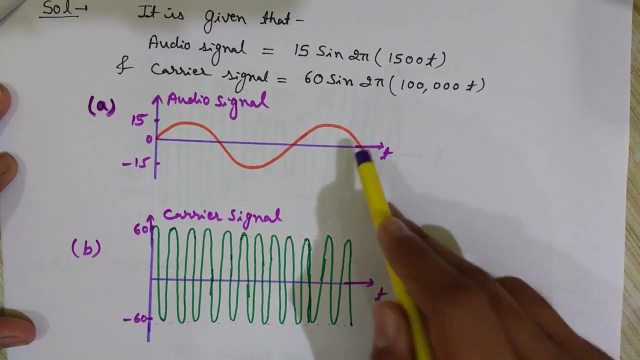 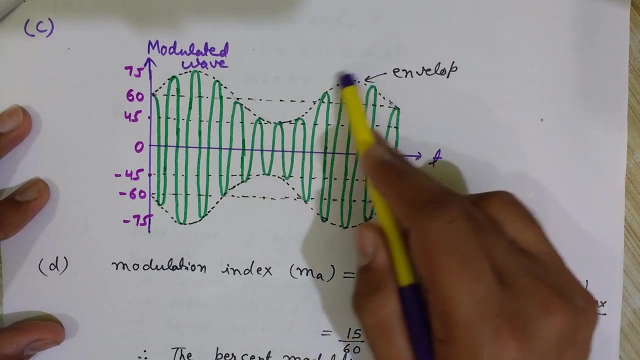 wave According to the instantaneous. instantaneous means at every instant. So the value present at every instant. So it's a shape. the peak of this carrier wave's amplitude will get the shape like this message signal, this audio signal. So look here, now the peak has taken the shape of its amplitude, of the message signal. 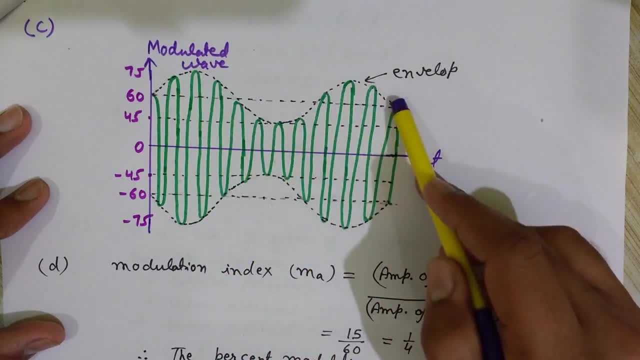 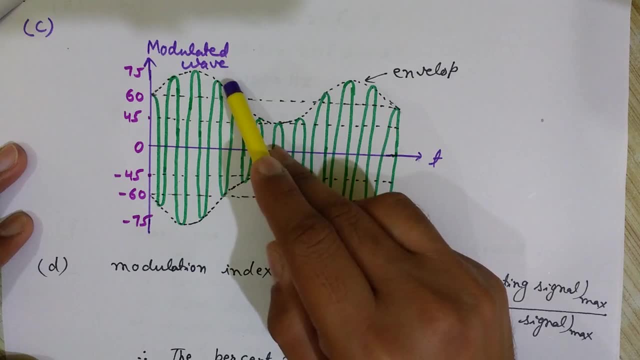 So here we have two bands. This is known as the upper side band. The whole information is present. We can retrieve the information present in the audio signal at the receiving end by the by this envelope. We call this as envelope. This is the envelope because this variation in the peak values of the amplitude of this 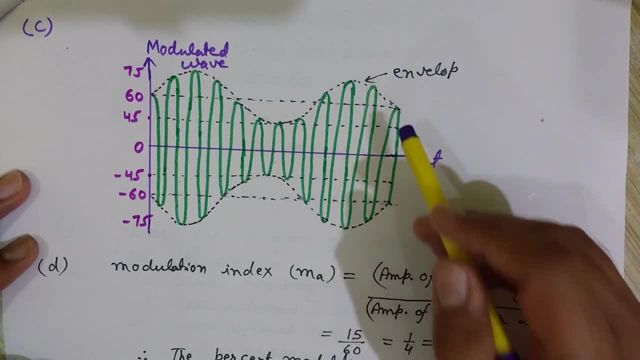 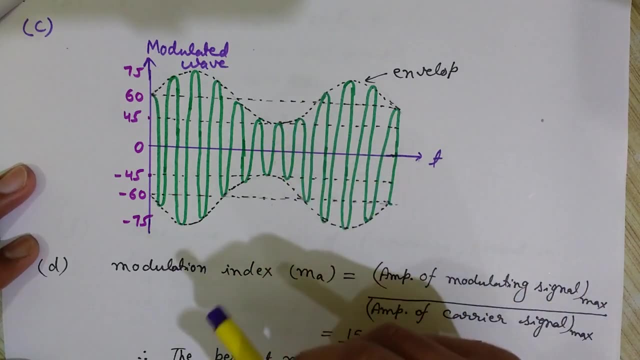 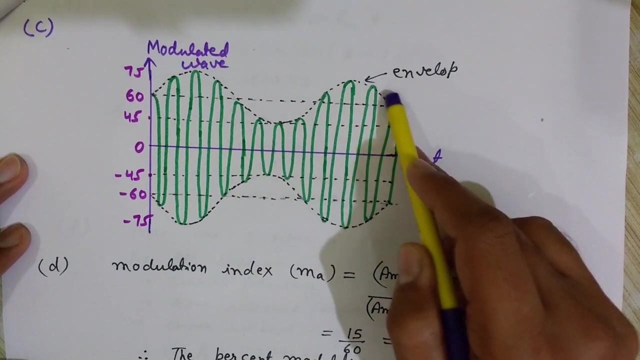 carrier has the whole information about this message signal. So we have: this is upper side band, this is lower side band and only one side band is enough to retrieve the full information about the message signal And how we have drawn this. you see, the variations are change in the amplitude of the carrier. 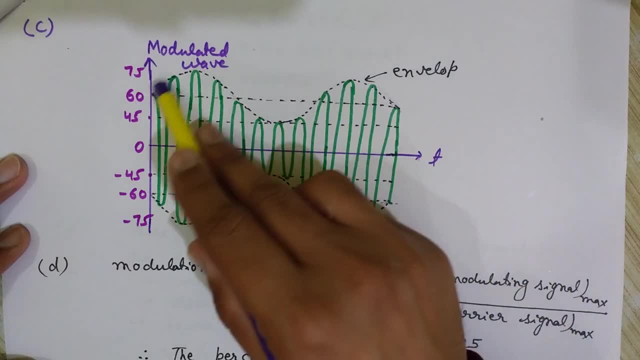 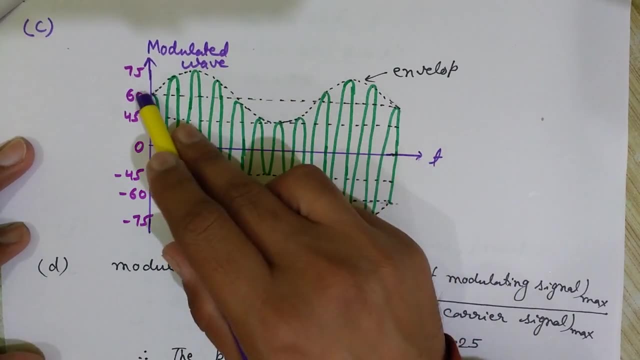 signal is according to the value of the amplitude of the message signal. So to draw this, you look at this, that this is the peak value when we draw the modulated signal, first, draw this line, this dotted line, and it is the 60 was the amplitude of the. 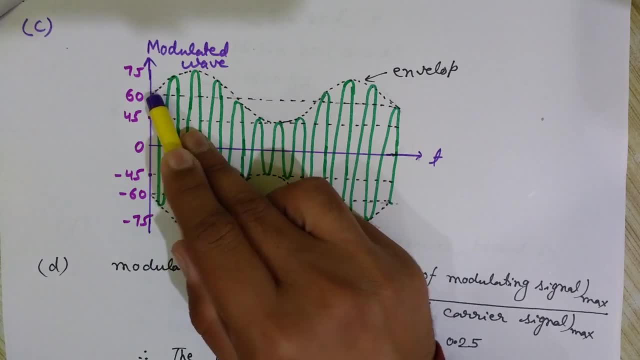 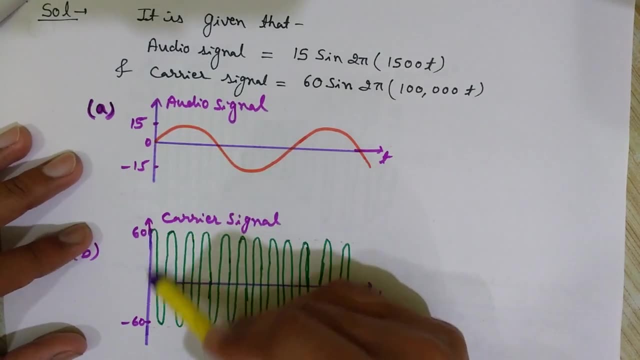 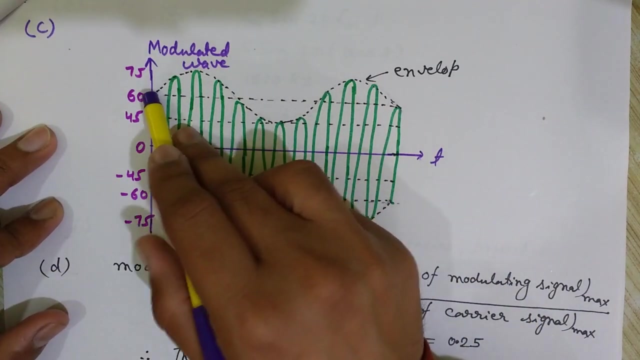 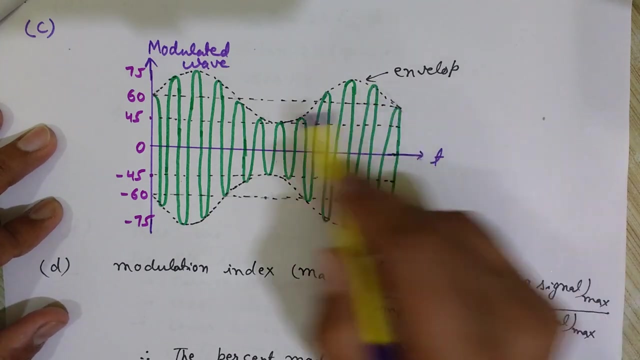 carrier wave, the peak value of the carrier wave. Look at this: 60.. 60. Was the amplitude of the carrier wave and 15- 15 is the amplitude of this message signal and 60 is the of that of carrier signal. So we to draw this, we take this as the axis and draw the shape of the message signal and 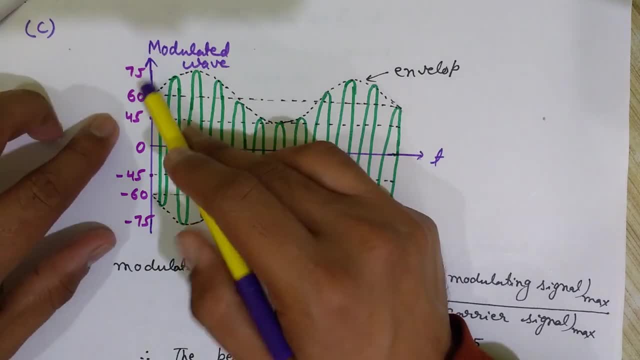 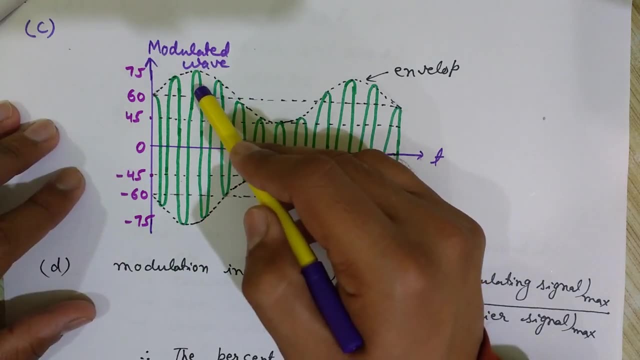 60 is the peak value of the carrier signal and you see here that 60. since this, this variation, is According to the message signal. so this: from the 60 value, or the peak value of carrier signal, it goes 15. 15 was the peak value of message signal. 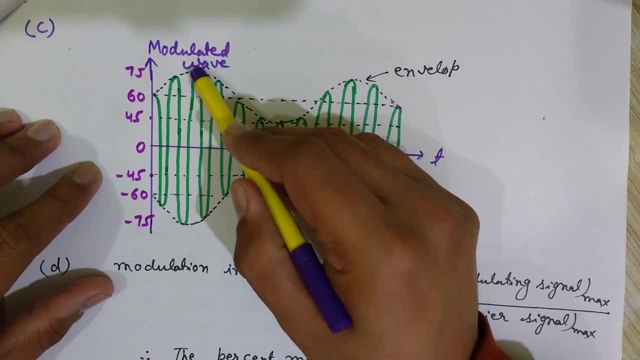 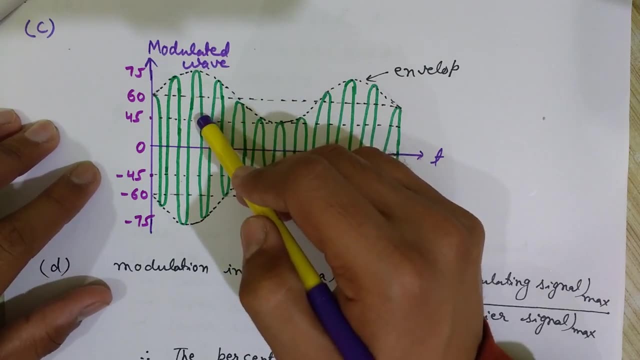 So this is the shape. So 15, 60 plus 15 and 60 minus 15. so 60 plus 15 is 75, 60 minus 15 is 45. So we draw this shape and in the identically we draw it on the negative side. 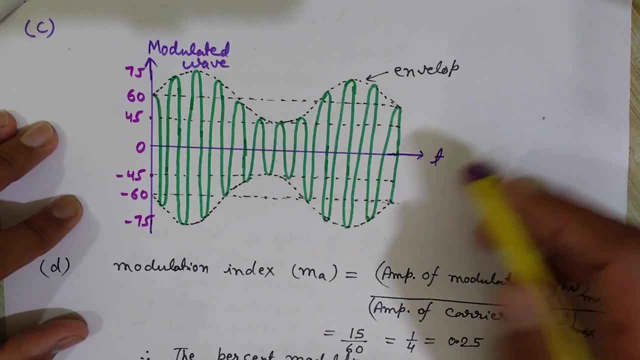 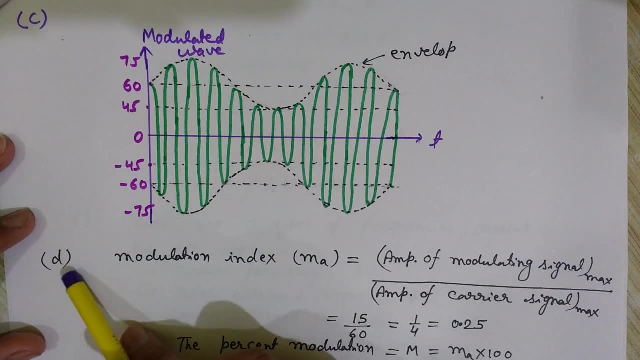 So this is the shape of the modulated waveform And we know We got this. and what is this importance? we can retrieve the modulating signal from this. Now, the fourth part of this problem is to find the modulation index and the percent modulation. 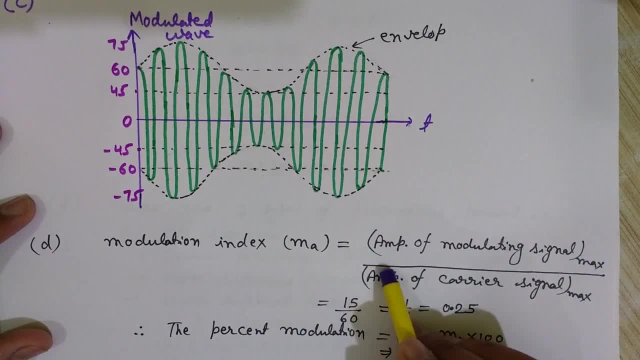 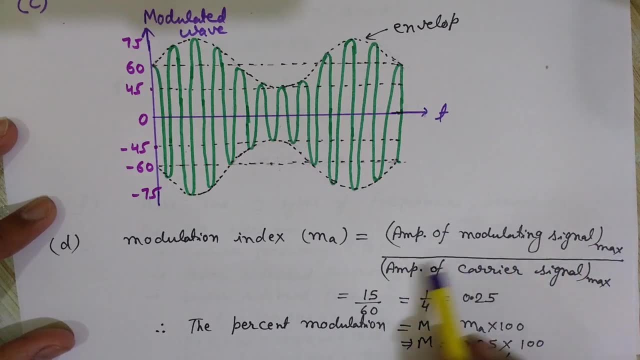 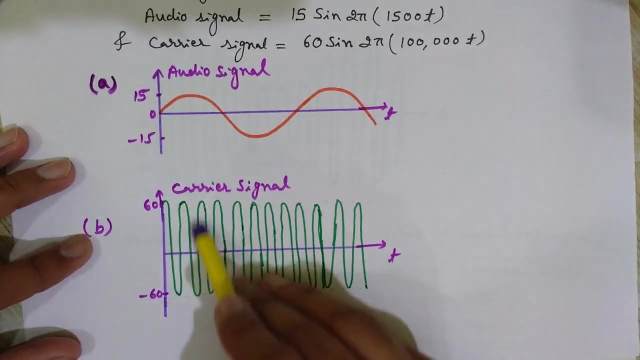 So the modulation index, by definition of modulation index for the amplitude modulation is the amplitude of the maximum amplitude of the modulating signal divided by the maximum amplitude of the carrier signal. Now we know both of these values. I told you that the maximum amplitude of the audio signal this is 15, and its value. 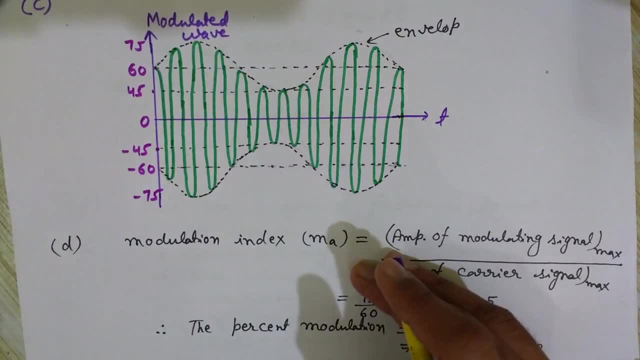 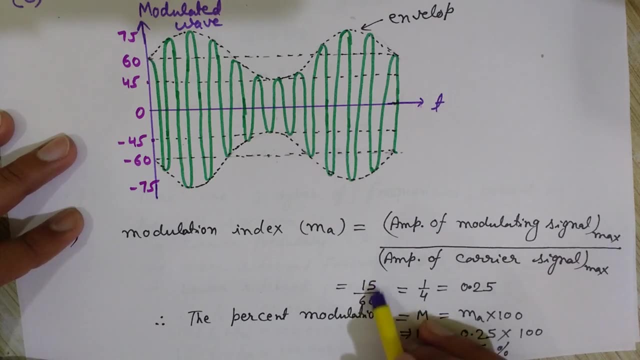 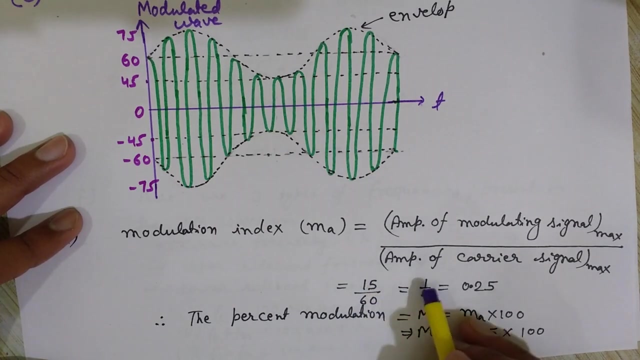 is 60 for the carrier, So we can easily find it 15 divided by 60.. So these are the ratio. This is modulation index is simply the ratio of amplitudes of a modulating signal, that is the message signal and the carrier signal. 15 by 60 comes out to be 1 by 4, so 0.25. and 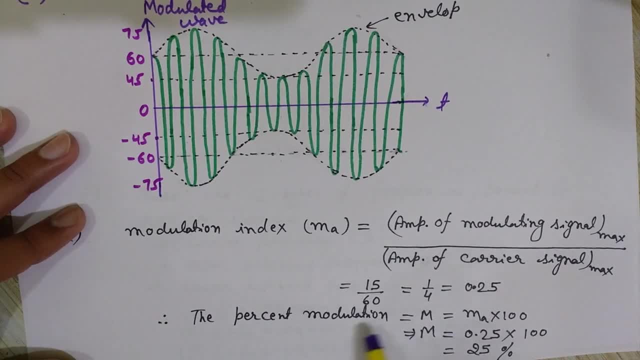 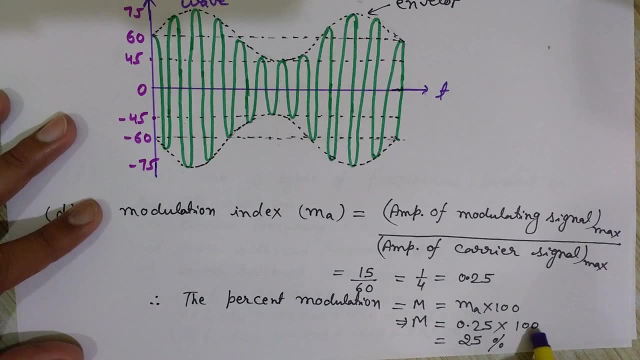 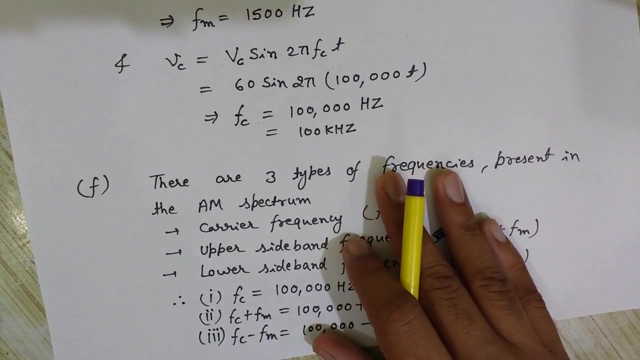 to calculate the percent modulation. it is in percent. So we just multiply this modulation index by 100.. So its value is simply 0.25 into 100. that is 25 percent. So 25 percent is the percent modulation. Now our next part, that is E part of this question, is: look at this: 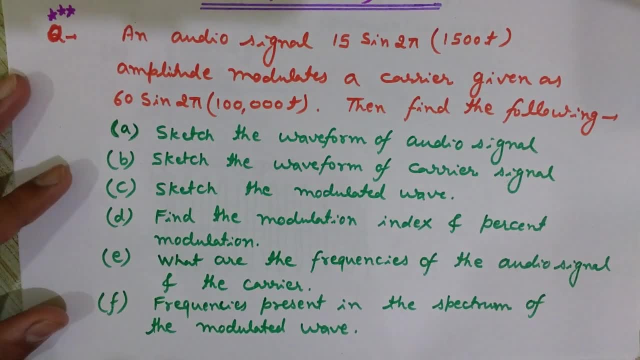 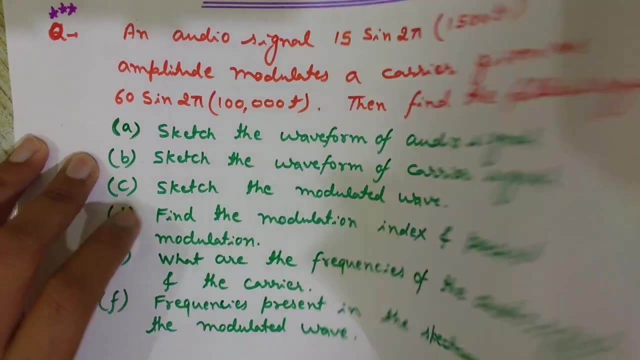 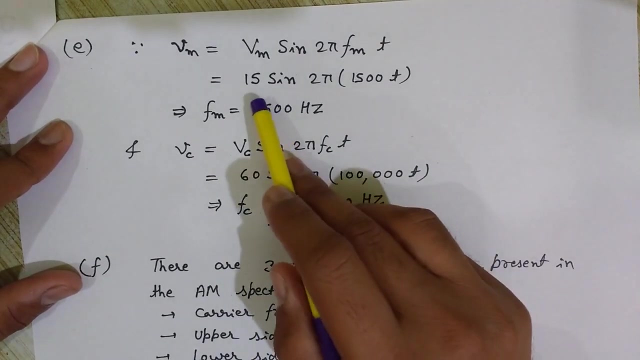 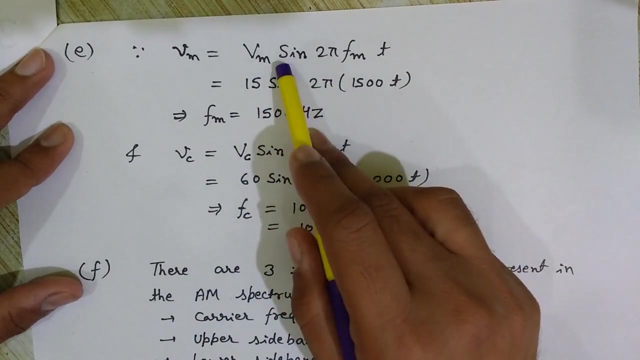 We have solved A, B, C and D parts of the question. E is: what are the frequencies of the audio signal And the carrier signal? So the frequency components that are present in the audio and carrier signal are, as we know, that 15 sine 2 pi, 1500 t is the given equation of audio signal and this is the standard. 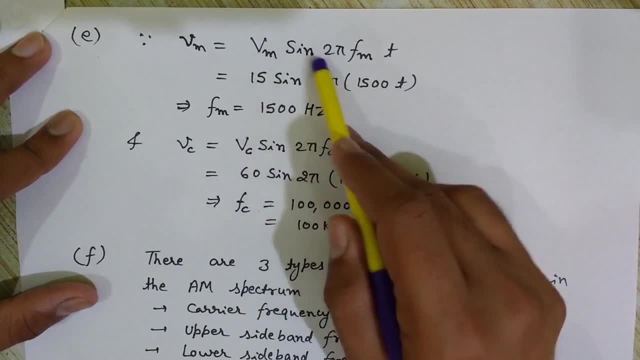 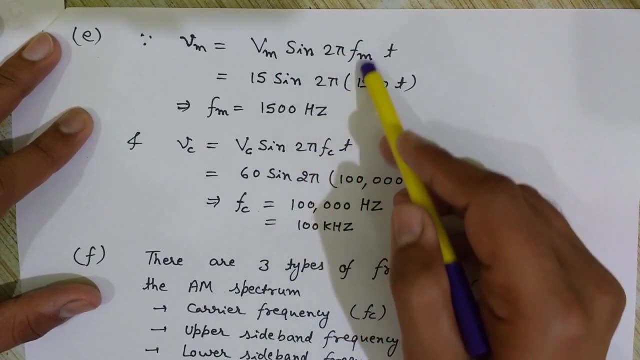 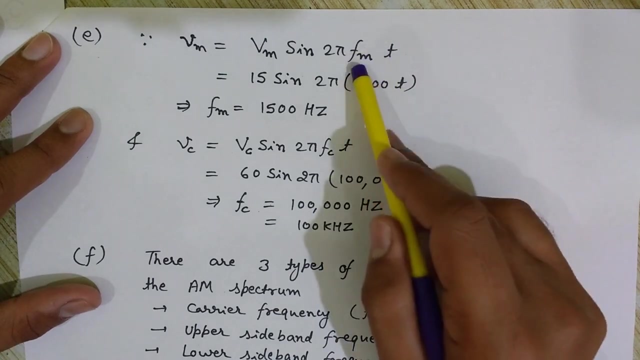 equation of the modulating signal V m sine 2 pi f m d. I have already discussed it earlier, just now that 2 pi. if you compare both of these, then this is the maximum. So the maximum amplitude 15 V m is equal to 15 and 2 pi f m. f m is the maximum frequency. 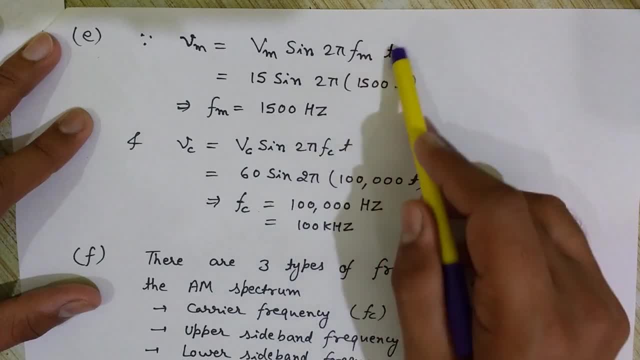 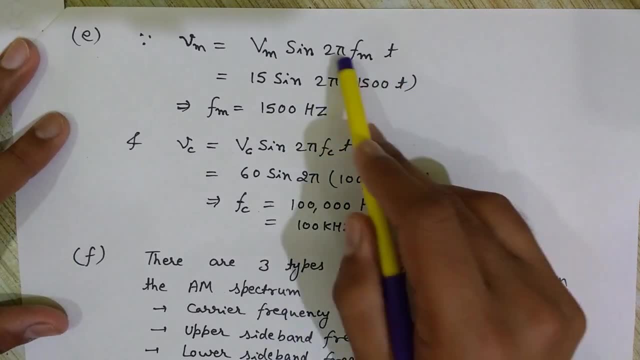 So corresponding to f m, it is 1500. just compare these. so 1500 is the 1500. hertz is the maximum frequency. This is 2 pi f m. 2 pi f m can also be written as omega t, V m sine omega t. 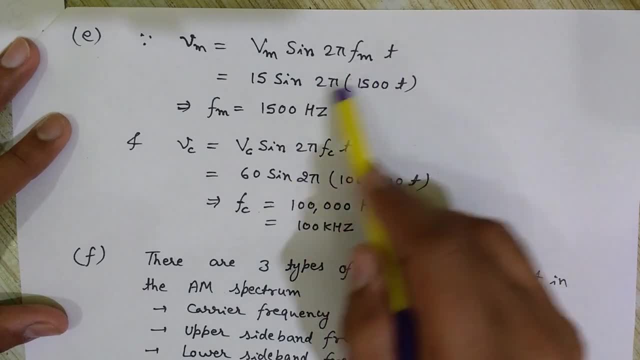 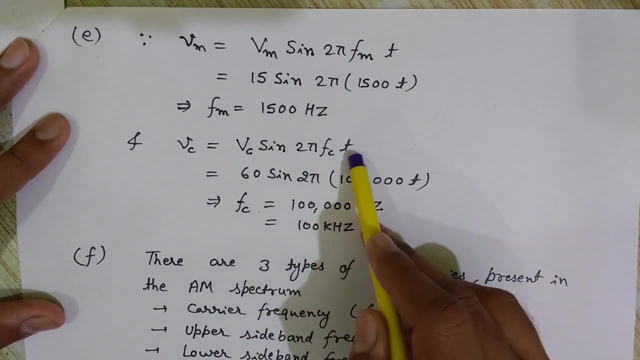 So omega would have been 2 pi 1500, but here we want to find the maximum frequency. it is 1500 hertz And exactly in the same way. this is the standard format: V, c, V, v, c, sine 2 pi, f, c, t for the carrier. 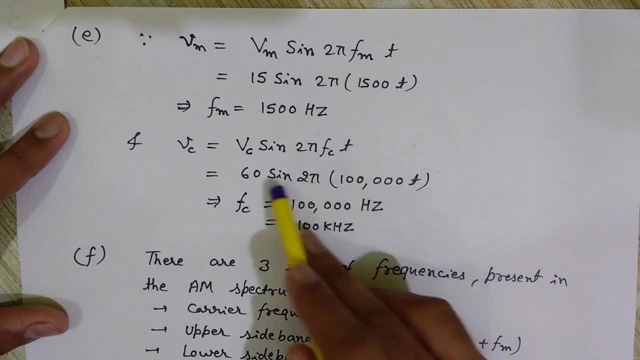 wave, and this is the equation for carrier wave So V c, maximum amplitude is 6 t and 2 pi f c. t 2 pi f c. So at the place of f c we have 100 k, 1 0, 0, 0 0 0.. 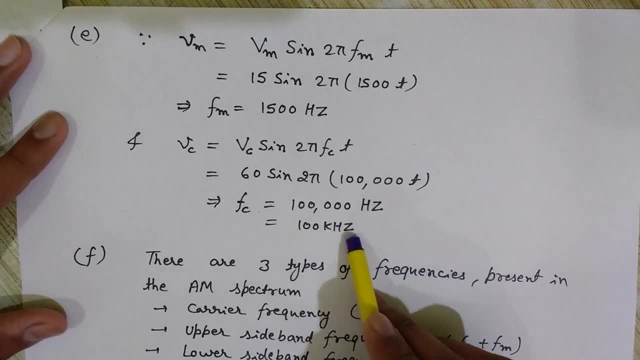 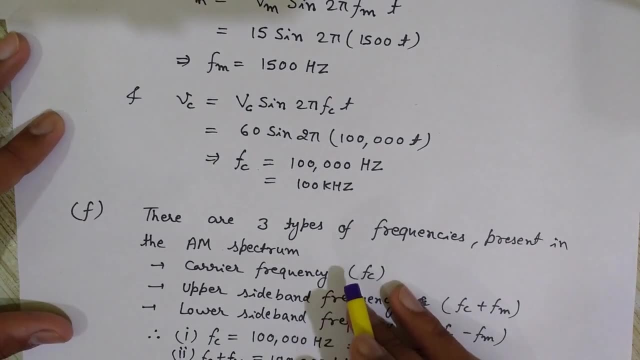 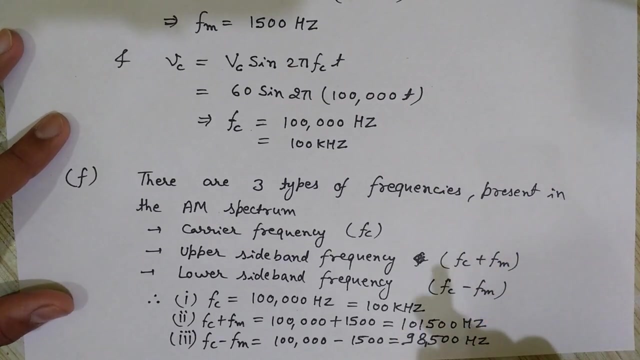 So this is the frequency. 100 kilohertz is the frequency. This is the maximum frequency present in the carrier signal. Now the last part, f part of the question is in the spectrum of amplitude modulation. this the amplitude modulation that we have seen. we need to find the frequency. 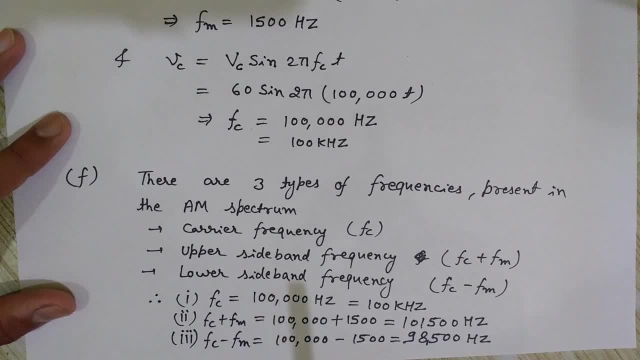 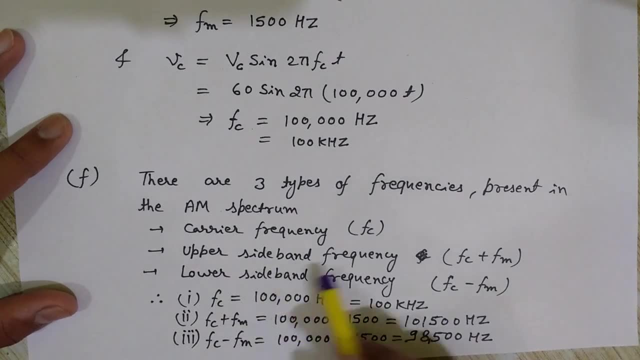 So actually there are three types of frequencies that are present in the amplitude modulation, amplitude modulated wave spectrum. First is the carrier frequency, Second one is the upper sideband frequency and third is the lower sideband frequency. So the first is the carrier frequency. 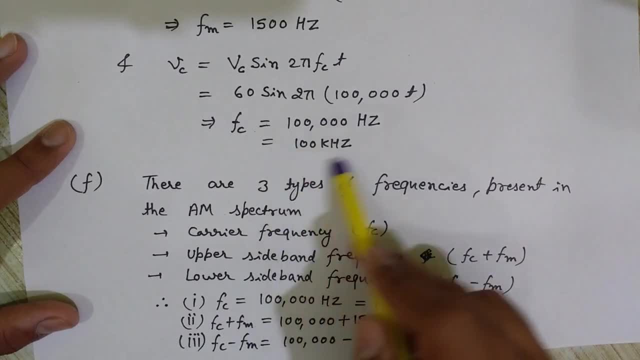 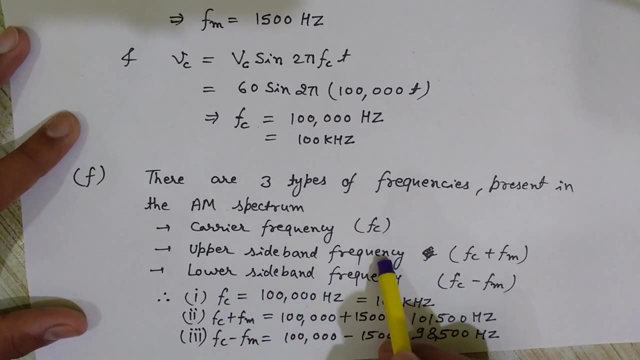 We have calculated the carrier frequency. it is 100 kilohertz. So 100 kilohertz, okay, 1 lakh hertz. and the second part is the upper sideband frequency. Upper sideband frequency is the frequency of the carrier plus the frequency maximum. 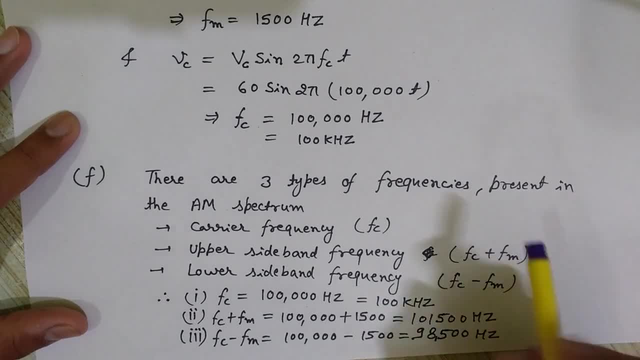 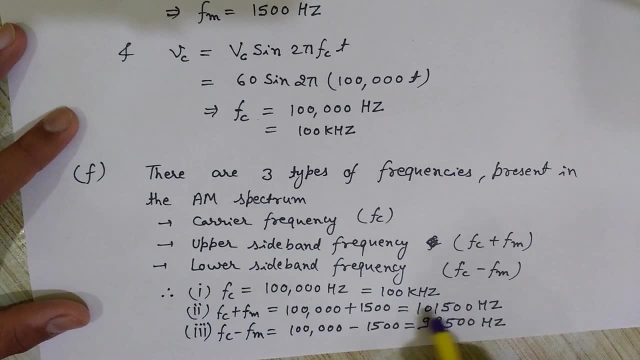 frequency present in the modulating signal, So f c plus f m. if you already know this f m, okay, f m. we have calculated and also know the f c. So f c plus f m, So 1, 0, 1, 5, 0. 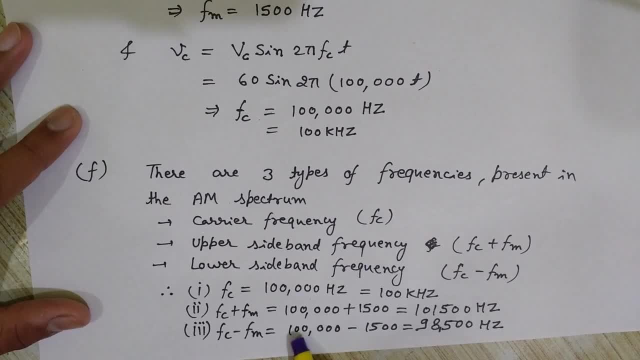 5, 0, 0 hertz and f c minus f m. f c minus f m means this: 100 k minus 1500.. So it is 98500 hertz. So all these frequencies, f c, f c plus f m and f c minus f m, three components of frequencies. 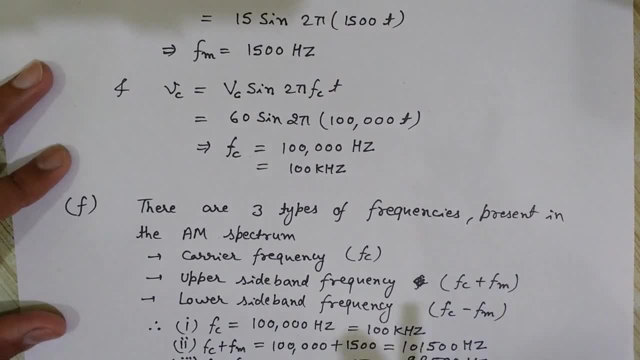 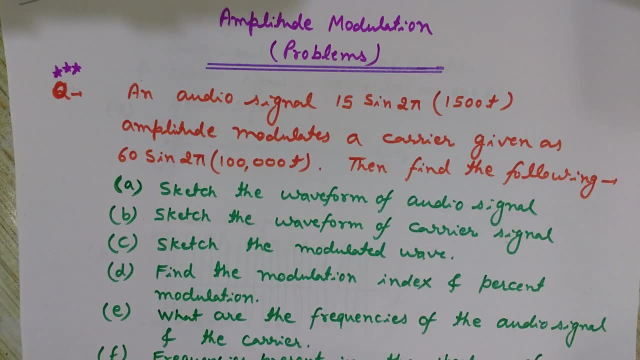 are present in the modulated signal: amplitude modulated signal. So these were the six parts of this problem and I'm sure you must have liked them. So in the next video we will see more problems On amplitude modulation, more solved problems and we'll see the basic concepts along with 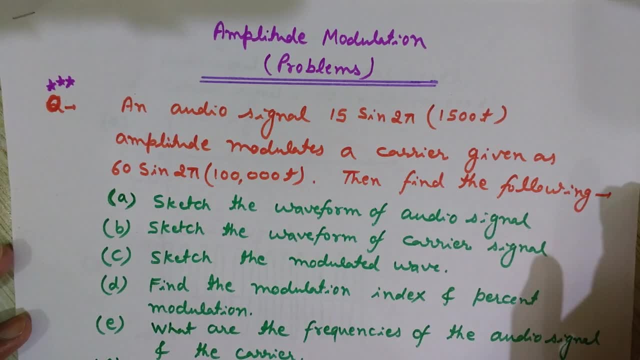 solving the problem. So, guys, see you in the next video with more such problems. Thanks for watching and if you have not subscribed to my channel, please don't forget to subscribe the channel. engineering made easy and like and share the video if you liked it. 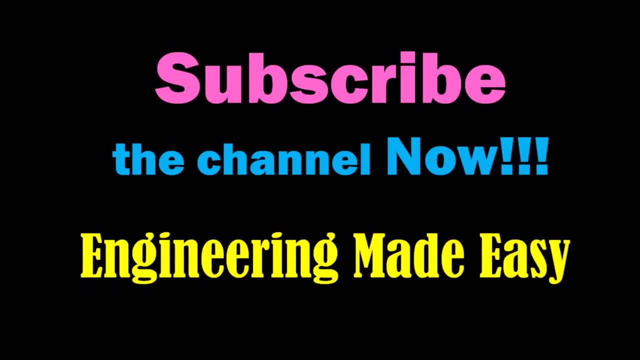 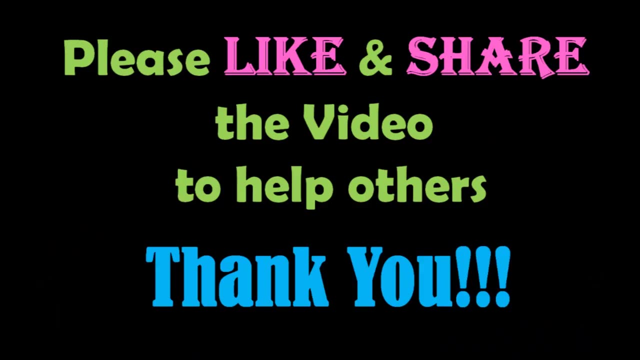 Thank you for watching. bye, bye, friends. for more such videos you can subscribe my channel- engineering made easy. And please don't forget to like and share the video if you liked it. For more detailed information, you can visit my blog. See you soon in the next video. till then, bye, bye.